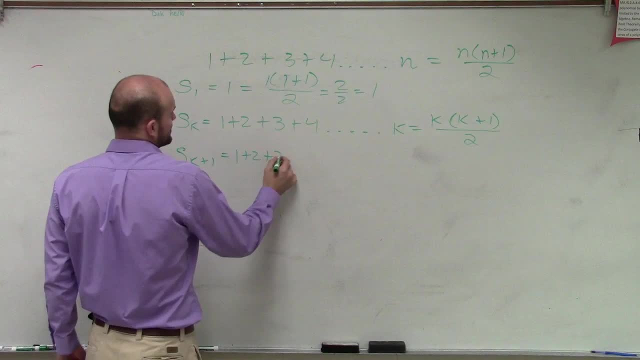 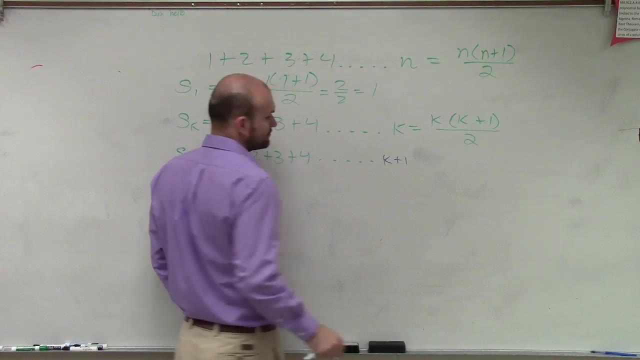 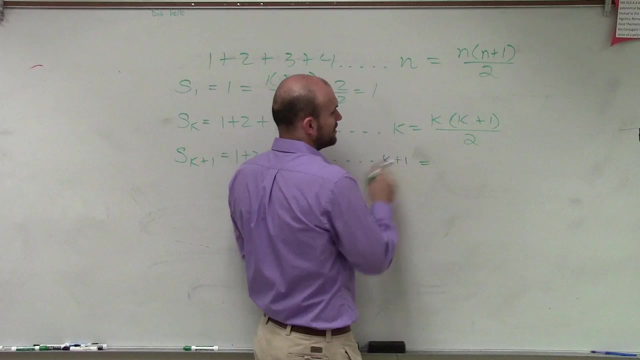 Sorry, s of k plus 1.. 1 plus 2 plus 3 plus 4. dot dot dot. The next term in the sequence is going to be k plus 1.. That now has to equal our. again I'm going to plug in k plus 1.. 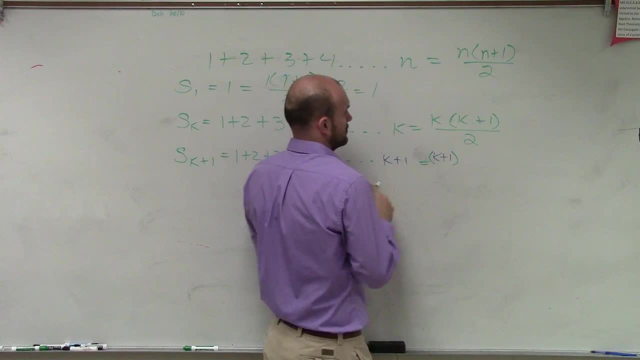 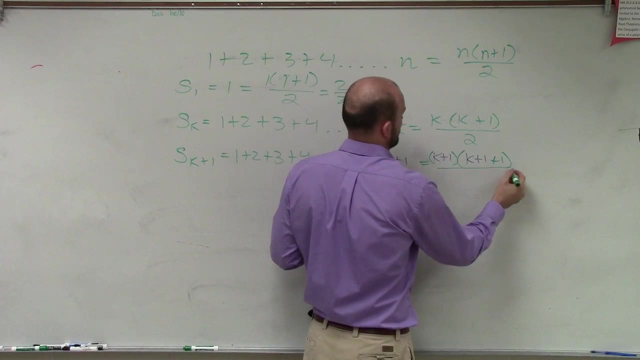 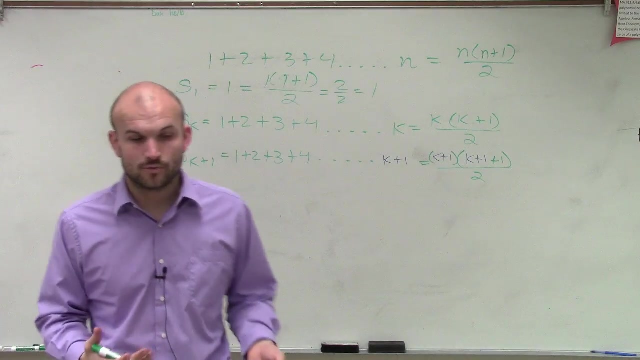 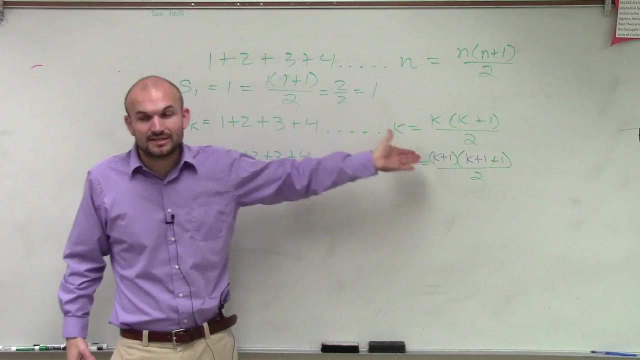 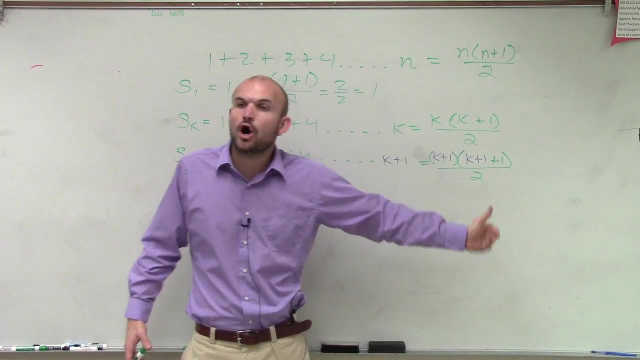 1.. Okay. So now to show that we have this working for us, we need to be able to show if, all right, if s of k plus the next term, next k plus 1 term, if that's equal to s of k plus 1, then it's going to be true for all of our values. 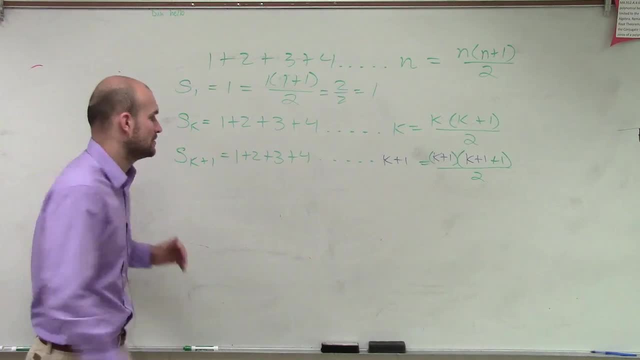 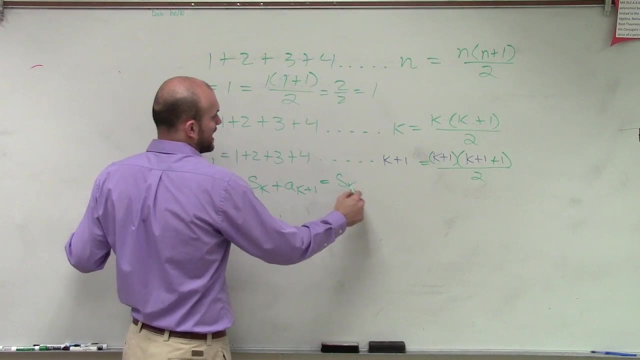 All right, And it's going to imply that all of our subsequent values on error will be true. So what I need to show is if s of k plus a of k plus 1 is equal to s of k plus 1.. So s of k plus 1 is right here. 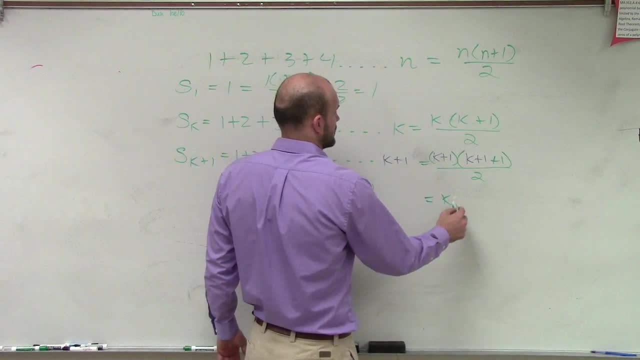 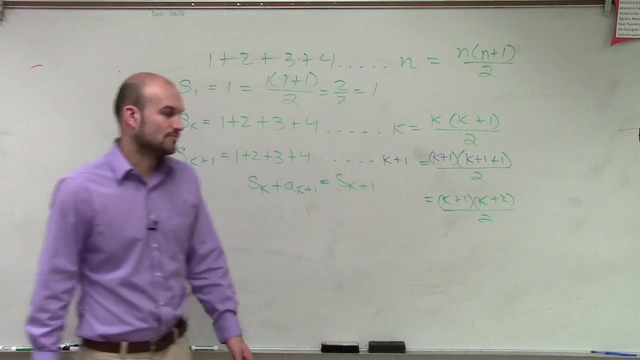 So what does s of k plus 1 simplify to k plus 1.. 1 times k plus 2 divided by 2.. So what I need to do is I need to take s of k. Well, what is s of k? 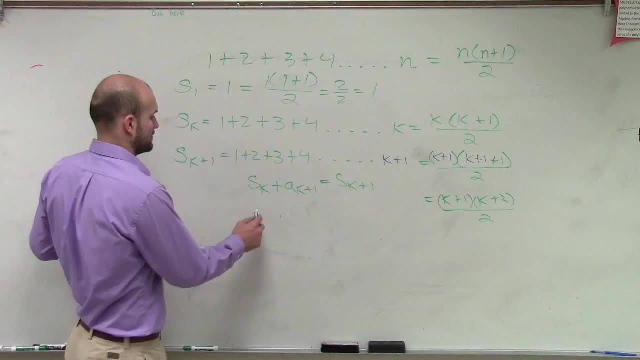 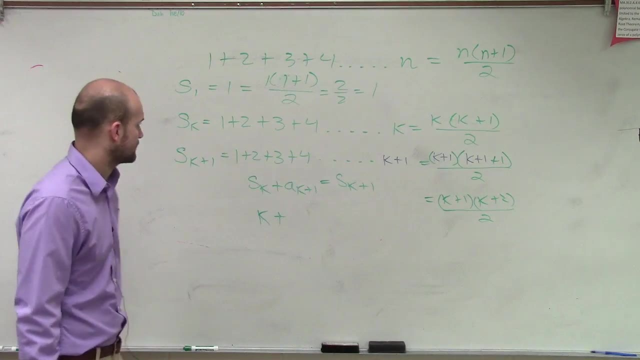 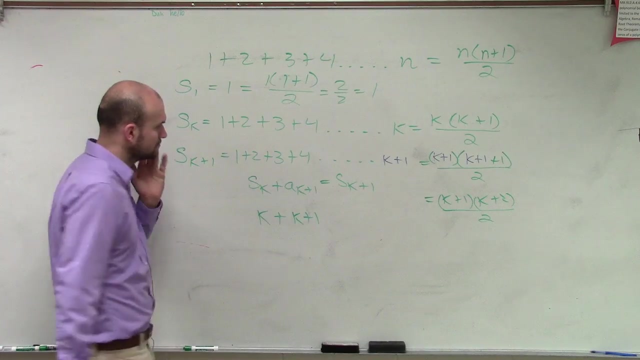 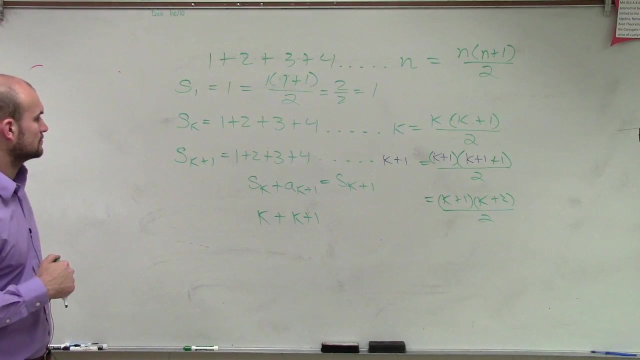 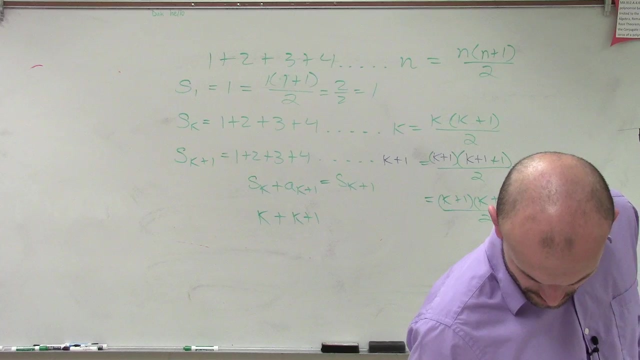 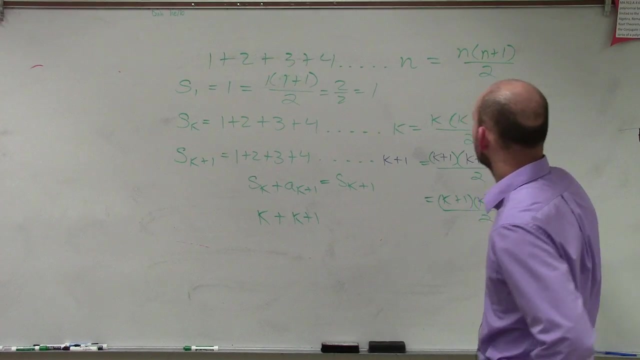 s of k is just k Plus a of k plus 1 is just k plus 1 over here s of k k. Oh wait, No, I'm sorry. What did I write? I'm sorry, S of k is not that. 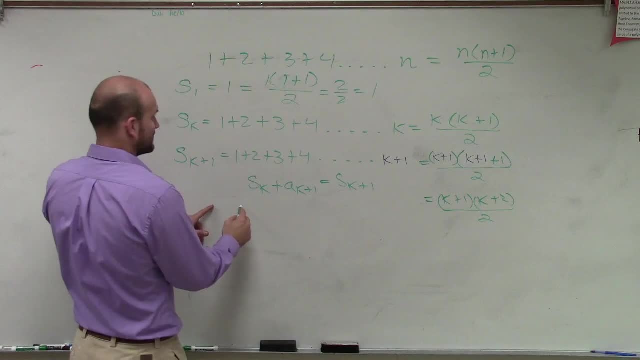 Jeez, I'm sorry, S of K is K right here. K times K plus 1 divided by 2. My bad Plus K plus 1.. Sorry, I was thinking like how am I going to get my fraction All right? So therefore we have this. 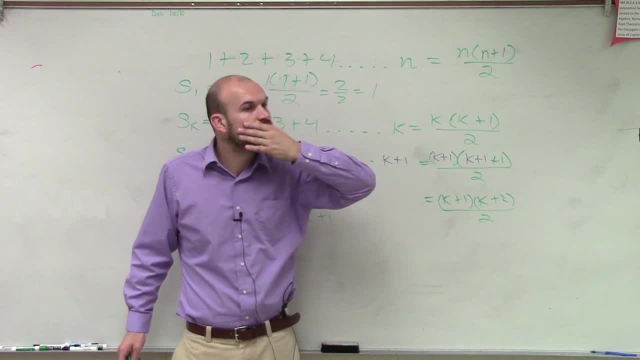 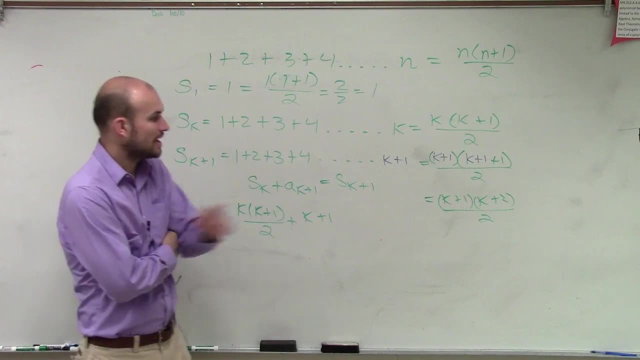 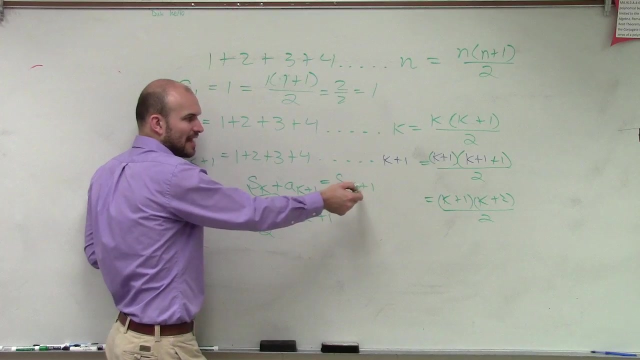 Do you guys understand? S of K is right here. Yes, Why doesn't K plus 1 equal? why doesn't it require me to use an equation that is equal? We are Right now. I'm just adding these two up. These two added up have to equal that. 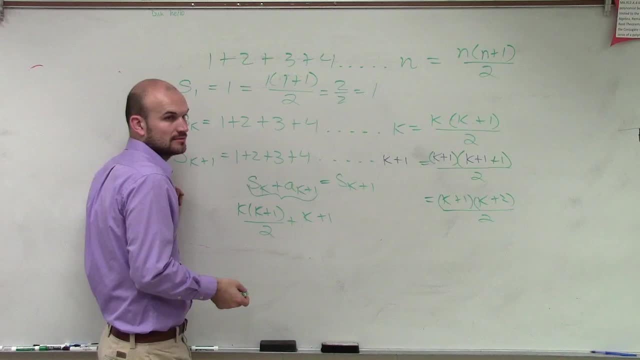 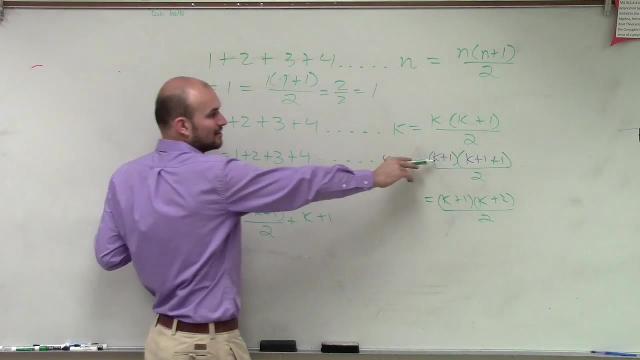 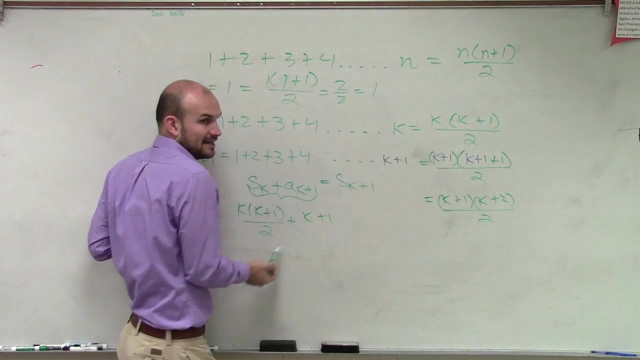 which is that, right there, We are saying this plus this has to equal that. So S of K plus 1 is right there. That has to be equal to ace of K plus 1 plus S of K. Oh, But like why? 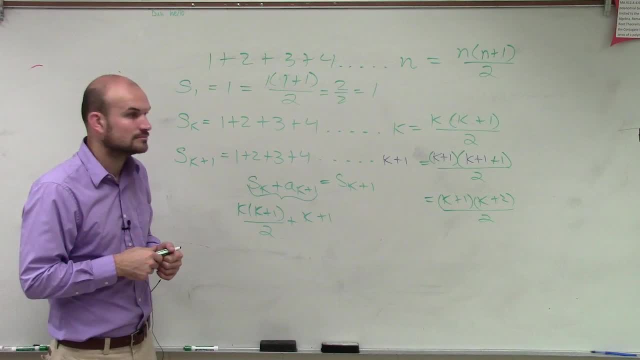 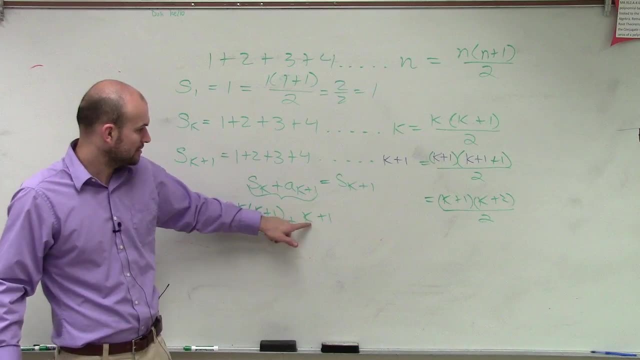 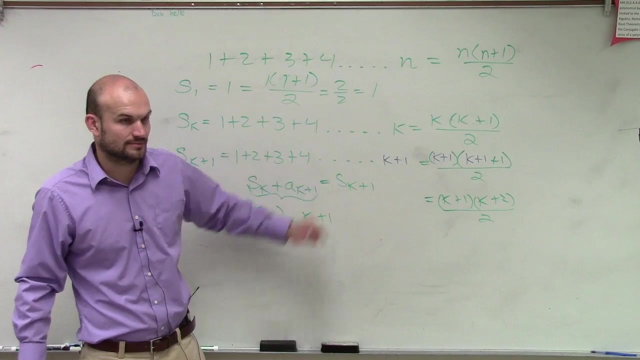 I am Ace of K plus 1 is right here. It's right there. I'm adding A of K plus 1 plus S of K And S of K plus A of K plus 1 has to equal S of K plus 1.. I am adding them. 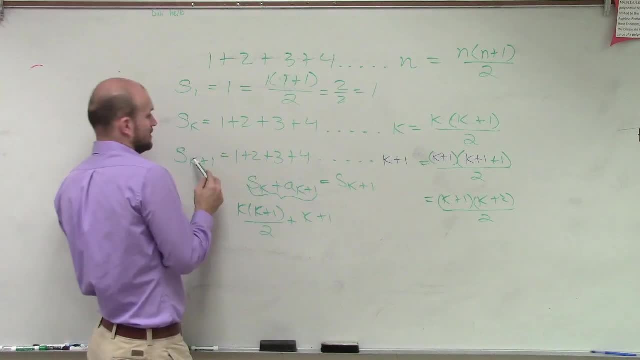 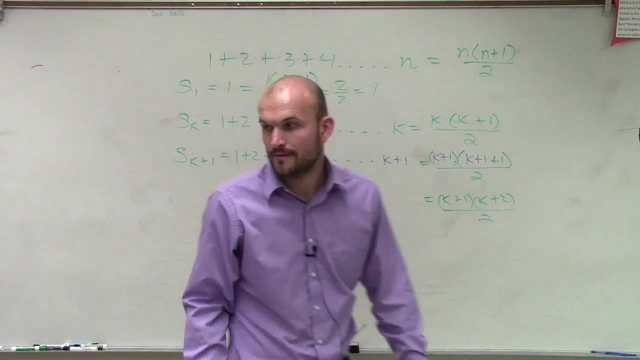 I'm taking S of K. S of K equals this. S of K plus 1 equals that. But it's S of K plus A of K equals this. S of K equals. this is what we're trying to prove. Question: What is ace of K plus 1?? 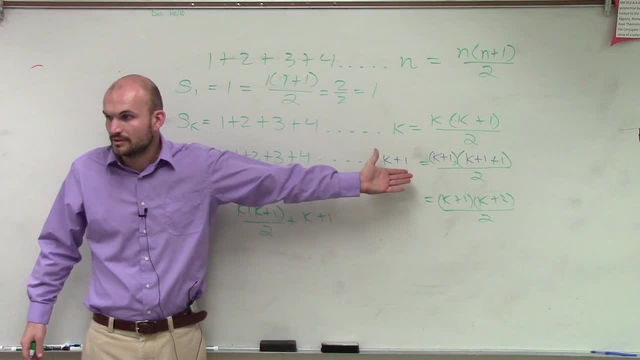 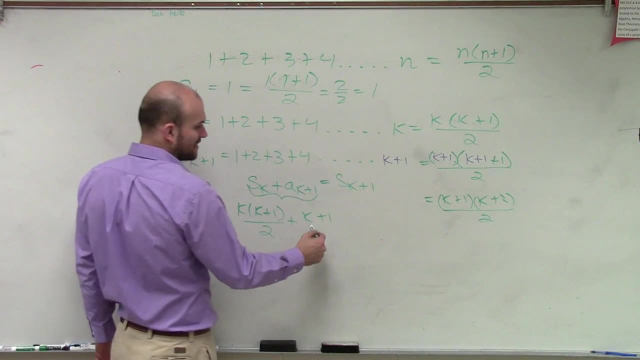 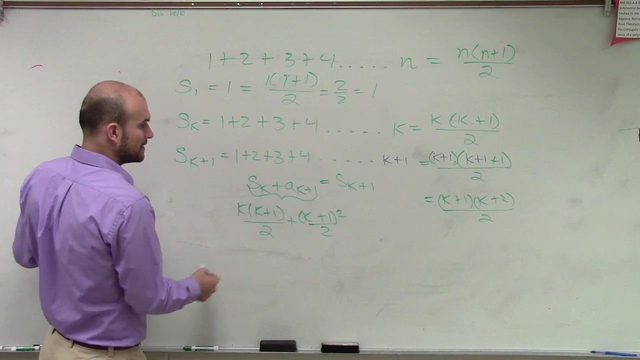 Ace, of K plus 1 is representing your next term. No, what is it? K plus 1.. Okay, So now if we have our two fractions, we need to get them together. So I need to multiply by 2 over 2.. So now we can get them to be together. So we'll have, let's see we can. 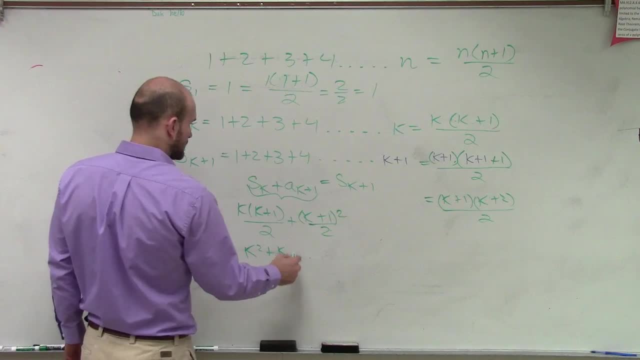 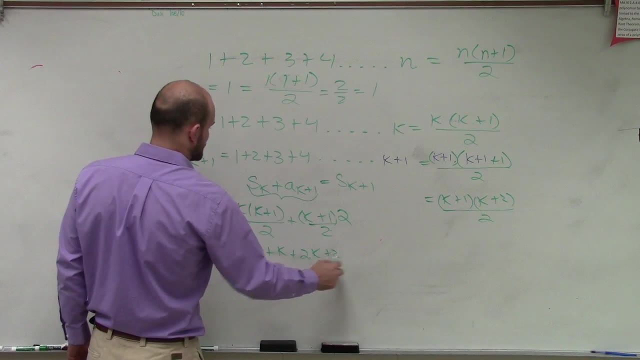 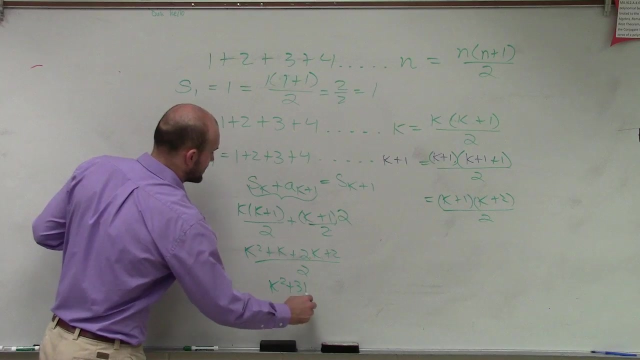 multiply this to give you K squared plus K plus S of K plus S of K. That's multiplied by 2, not square root of 2.. Plus 2K plus 2 all over 2.. Well, here I can add this up into K squared plus 3K plus 2 over 2.. Then, ladies and gentlemen, what? 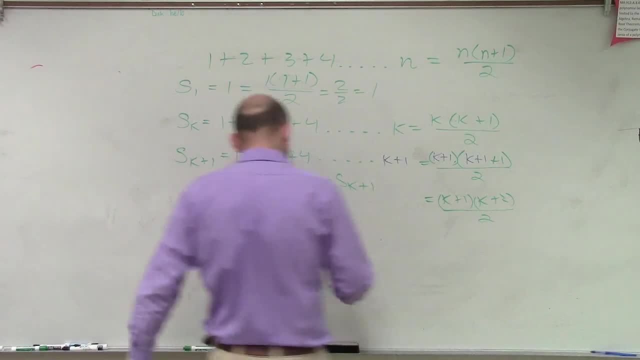 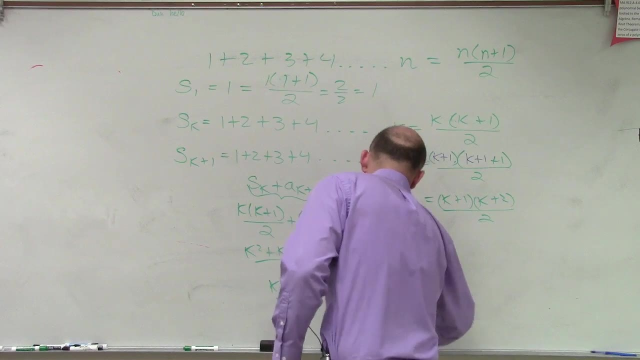 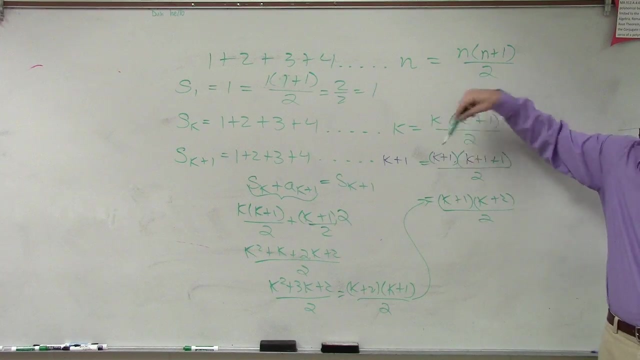 you can see, is this can be factored right. This can be factored into K plus 2 times K plus 1.. Which you guys can now see is exactly the same as S of K plus 1.. So therefore it's: